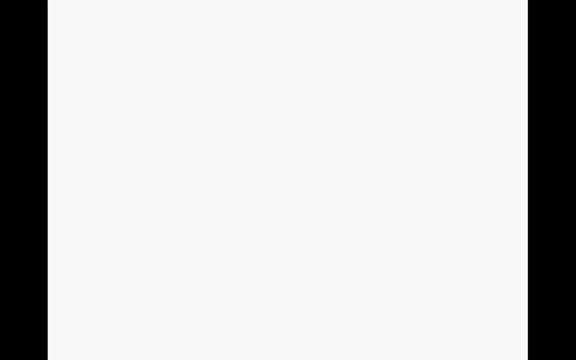 in writing. the decimal expansion of the fraction- So we have 5 eighths- is equal to 5 times 10 to the third factor, over 8 times 1 over 10 to the third power. When we do that, we have 5000 over 8 times 1 over 10 to the third power. 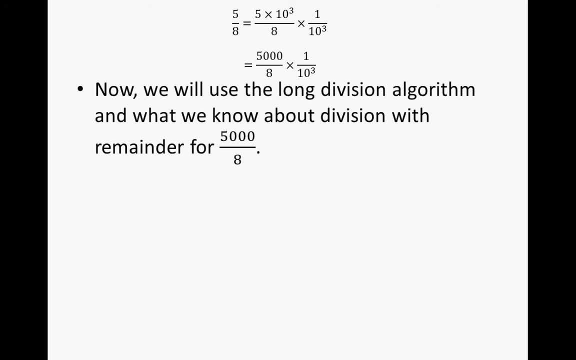 Now we will use the long division algorithm and what we know about division with the remainder for 5000 eighths. So 5000 eighths times 1 over 10 to the third power is represented division-wise as 625 times 8 plus 0.. 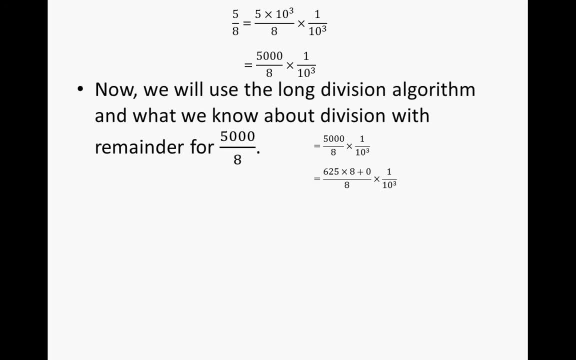 0 over 8 times 1 over 10 to the third power. We can separate this by making this an addition problem. So 625 times 8 over 8 plus 0 over 8 times 1 over 10 to the third power. 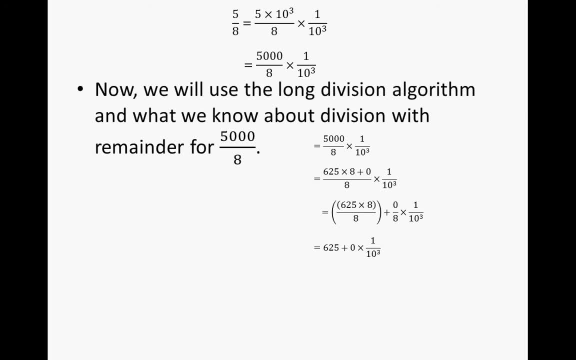 That leaves us with 625 plus 0 times 1 over 10 to the third power And 625 times 1 over 10 to the third power is 625 over 10 to the third power. This is 625 thousandths. 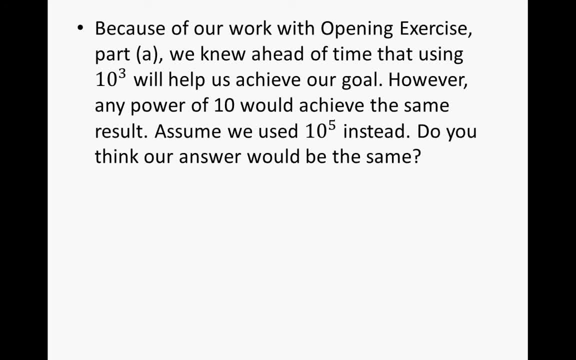 Because of our work with the opening exercise, Part A, we knew ahead of time that using 10 to the third power will help us achieve our goal. However, any power of 10 would achieve the same result, Assume we use 10 to the fifth power instead. 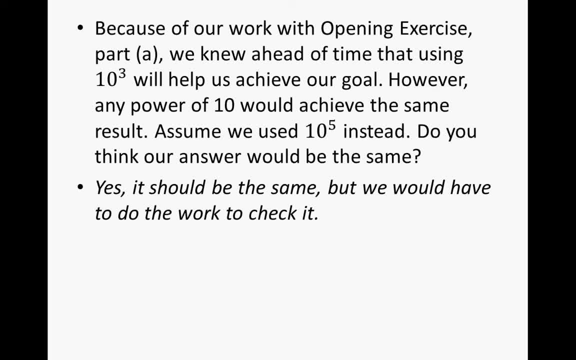 Do you think our answer would be the same? Well, yes, it should be the same, but we would have to do the work to check it. So let's verify that our result would be the same if we use 10 to the fifth power. 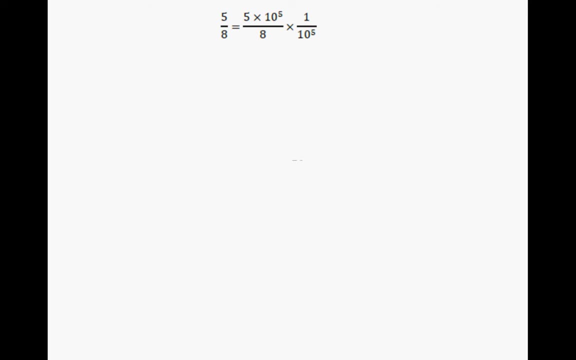 So, starting off again and multiplying by 10 to the fifth power, And then also We have 5200 times 1 over 10 to the fifth power. We have 500,000 over 8 times 1 over 10 to the fifth power. 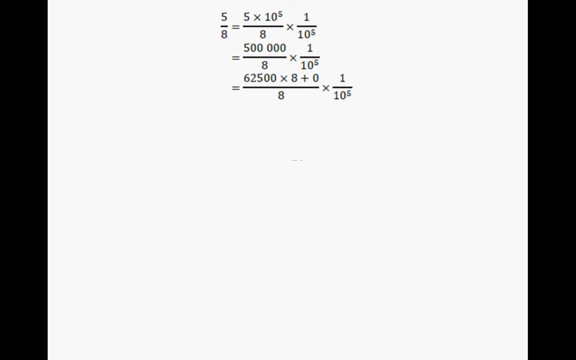 This becomes 62500 times 8 plus 0 over 8 times 1 over 10 to the fifth power. Separating this into addition, this would be 62500 plus 0 over 8 times 1 over 10 to the fifth power. 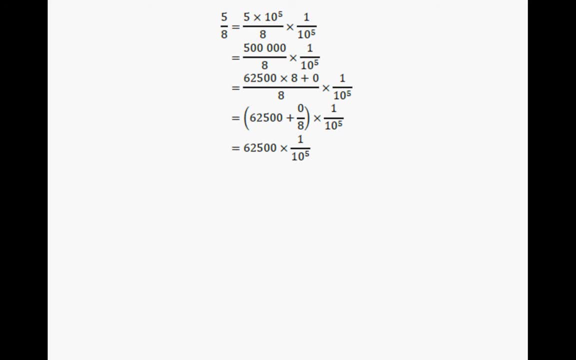 Which is 62500 times 1 over 10 to the fifth power, Which again is 62500 over 10 to the fifth power, And that is 62500 hundred thousandths, Which again is the same as 625 thousandths. 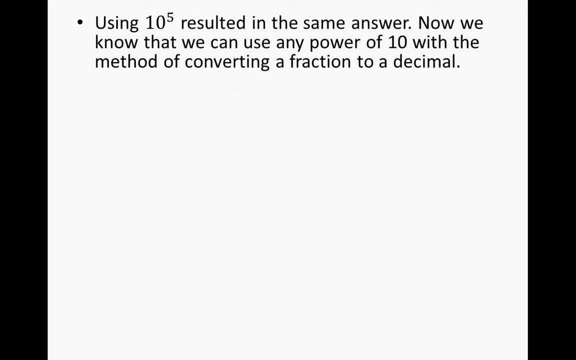 So using 10 to the fifth power resulted in the same answer. Now that we know we can use any power of 10 with the method of converting a fraction to a decimal, This process of selecting a power of 10 to use is similar to putting zeros after the. 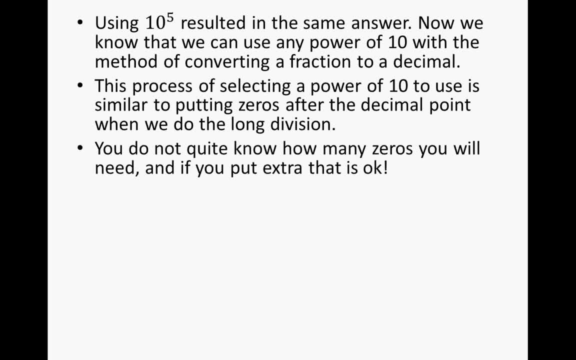 decimal point. when we do long division, You do not quite know how many zeros you will need, And if you put an extra one, that is okay. Using lower powers of 10 can make things more complicated. It is similar to not including enough zeros when doing the long division. 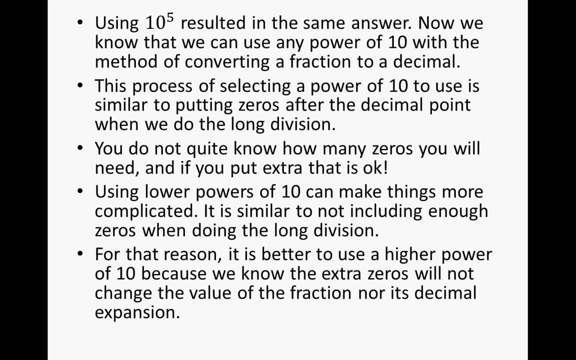 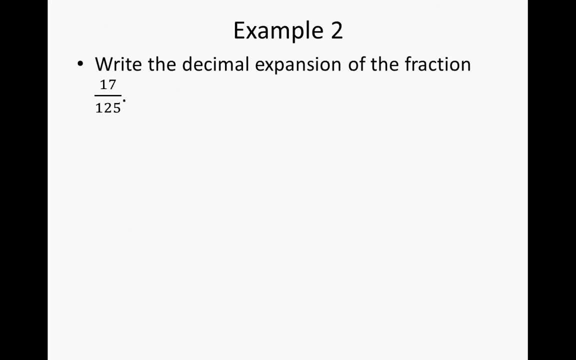 For that reason it is better to use a higher power of 10, because we know the extra zeros will not change the value of the fraction nor its decimal expansion. Alright, let's take a look at example 2.. Write the decimal expansion of the fraction: 17 over 125.. 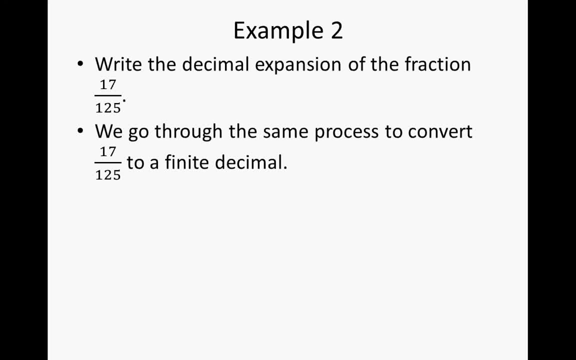 We go through the same process to convert 17 hundred and twenty-fifths to a finite decimal. We know from the opening exercise that 17 over 125 is a finite decimal. We know from the opening exercise that 17 over 125 is a finite decimal. 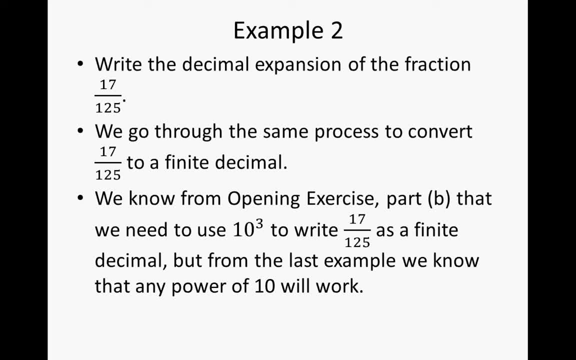 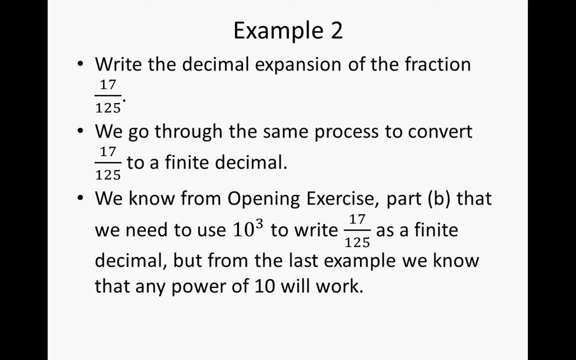 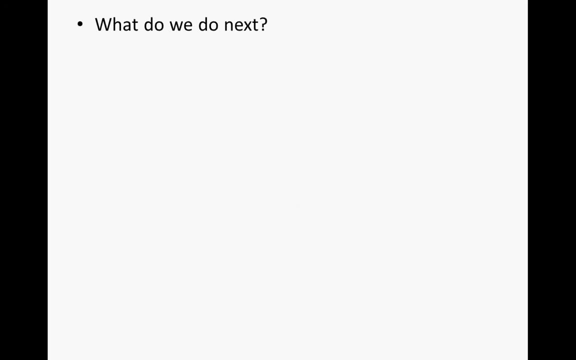 From the last example we know that any power of 10 will work. So 17 hundred and twenty-fifths is the same as 17 times 10 to the third, over 125 times 1 over 10 to the third power. 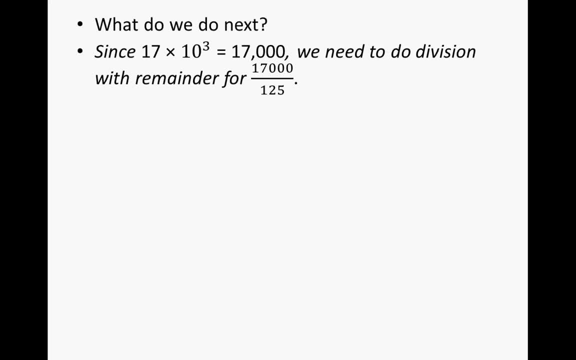 What do we do next times? 10 to the third power, 17,000. we need to do division with the remainder for 17,000 over 125.. So do the division with the remainder and write the next step. Go ahead and pause the video until you are done. You should have 17,000 over. 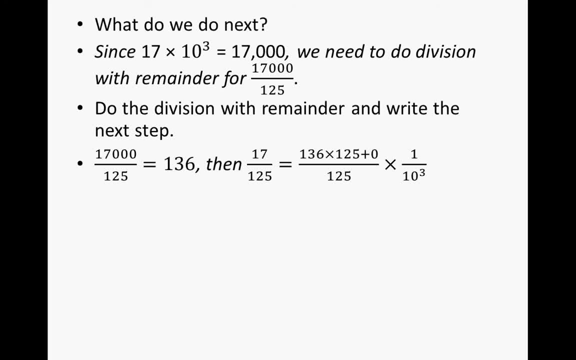 125 is 136. Therefore, 17,125 is 136 times 125 plus 0 over 125 times 1 over 10 to the third power. Now let's finish the work and write 17,125 as a finite decimal, So 136. 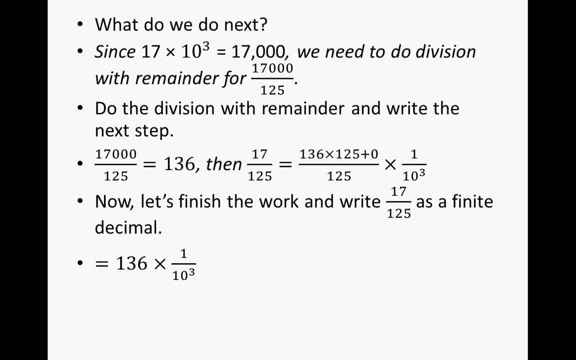 is times 1 over 10 to the third power, which is 136 times 1 over 10 to the third power, 36 over 10 to the third power, which is 136 thousandths. All right, example 3.. Write the: 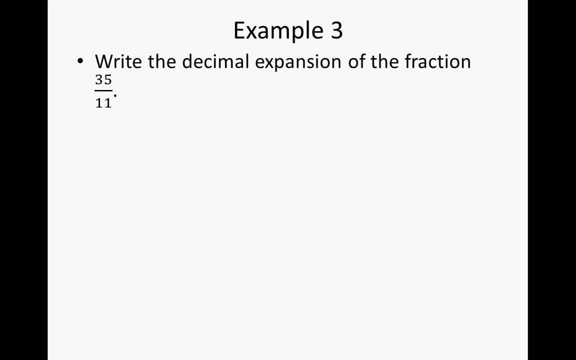 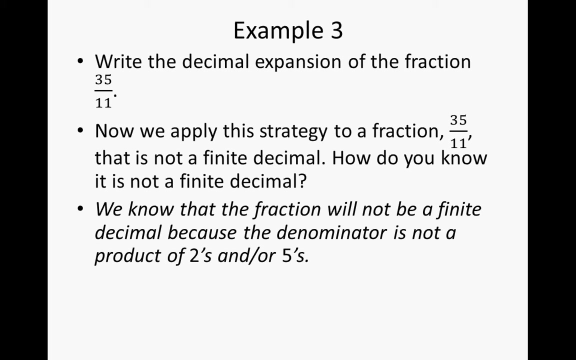 decimal expansion of a fraction: 35 elevenths. Now we apply this strategy to a fraction- 35 elevenths. that is not a finite decimal. How do you know that it's not a finite decimal? Well, you know that the fraction will not be finite decimal because a denominator is. 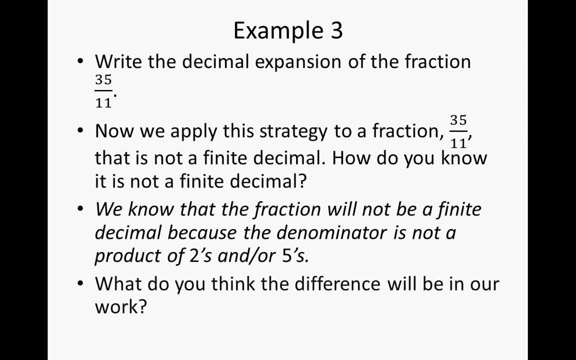 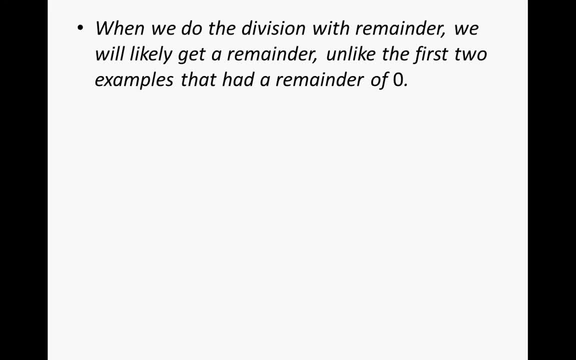 not a product of 2s and or 5s. So what do you think the difference will be in our work? Well, when we do the division with the remainder, we will likely get a remainder, Unlike the first two examples that had a remainder of 0.. 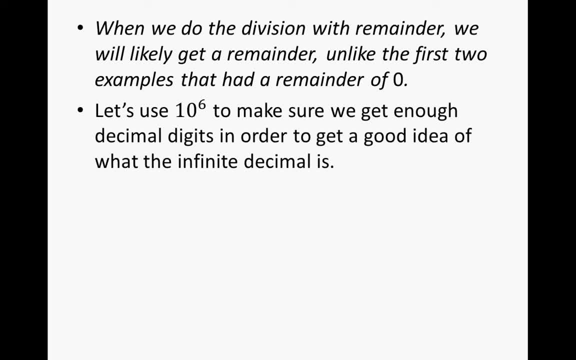 So we are going to arbitrarily use 10 to the 6th power to make sure we get enough decimal digits in order to get a good idea of what the infinite decimal is. We can pick any power of 10, but we don't want to make the number too cumbersome, so maybe 10 to the 10th power. 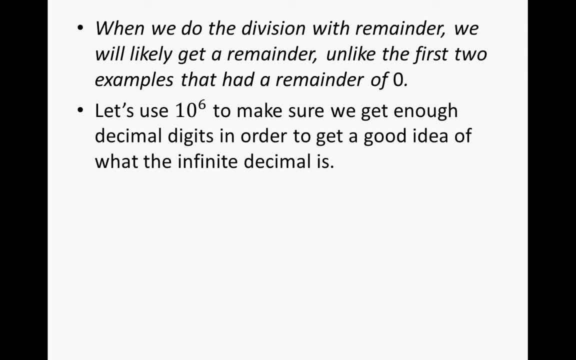 would be too much and, like we mentioned before, we don't want to pick too few. so 10 to the third or fourth might not be enough. So 10 to the 6th is just an arbitrary number we have picked and that's kind of a number in the middle part. that should give us what we 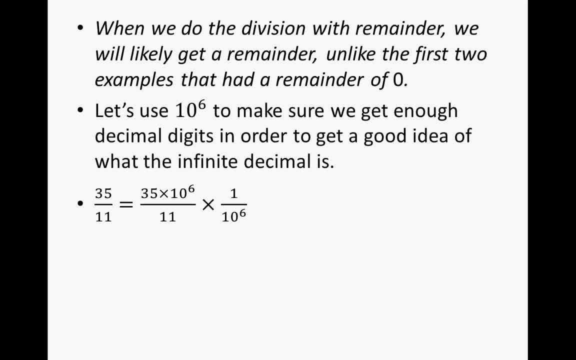 need. So 35 over 11ths is equal to 35 times 10 to the 6th power over 11,, which is times 1 over 10 to the 6th power. So what do we do next? Well, since 35 times 10 to the 6th, 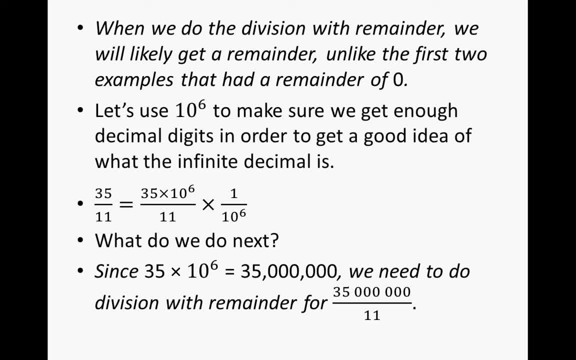 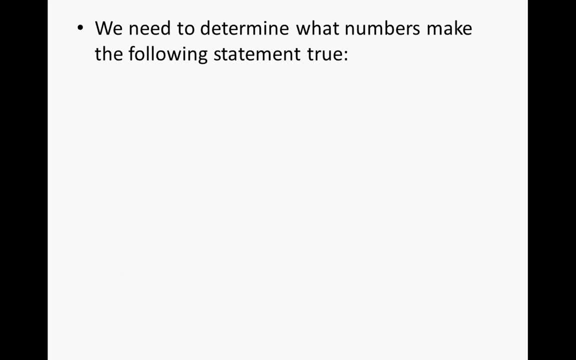 power is 35 million, we need to do division with remainder for 35 million divided by 11.. So we need to determine what numbers make the following statement true: 35 million is equal to some number times 11 plus some number. Well, that would be 3,181,818,. 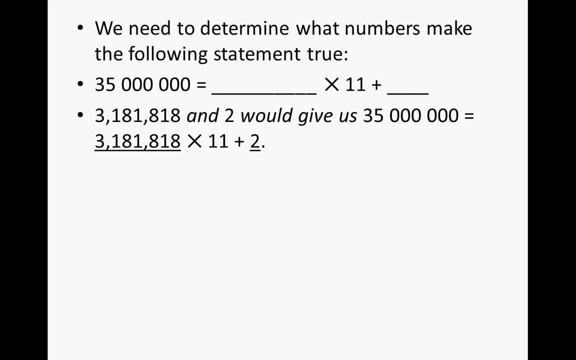 and 2 would give us 35 million. So it would be: 35 million is equal to 3,181,818 times 11 plus 2.. So with this information we can continue the process. So 35-elevenths is the same as 3,181,818 times 11 plus 2 over 11 and multiplied that. 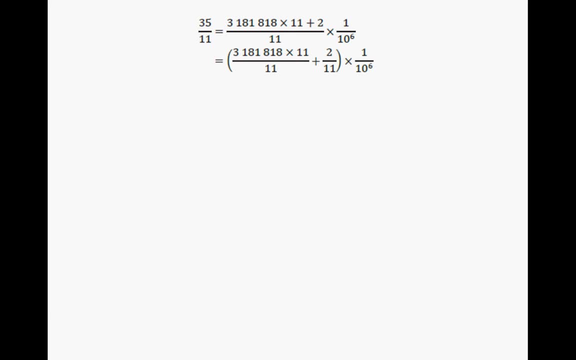 by 1 over 10 to the 6th power. So using this is an addition problem. we get 3,181,818 times 11 over 11 plus 2-elevenths, and then by 1 over 10 to 6th power. Pump it out the other way. Okay. Now we've got 13,101,181,181,810 times 11, over 11 plus 2-elevenths, and thencan I use this one to incorporate the sum? Okay? 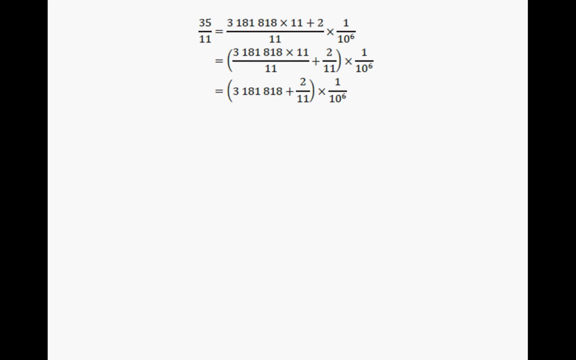 So what we're doing here in this problem is that we just multiply anything by one. So let's see what is given in the expertise power. Well, now that, since we have that, that cancels out, and we have 3,181,818 plus 2 11ths. 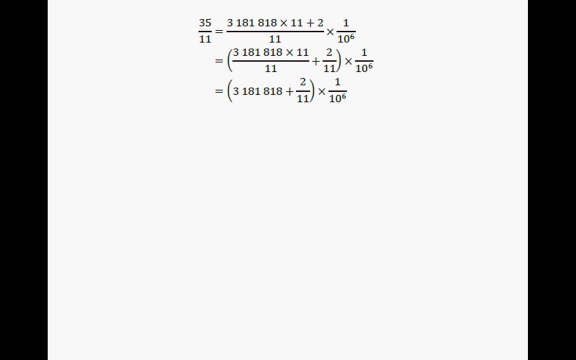 times 1 over 10 to the 6th power. Using distributive property. we're going to multiply both terms by 1 over 10 to the 6th power, So we have 3,181,818 times 1 over 10 to the 6th power. 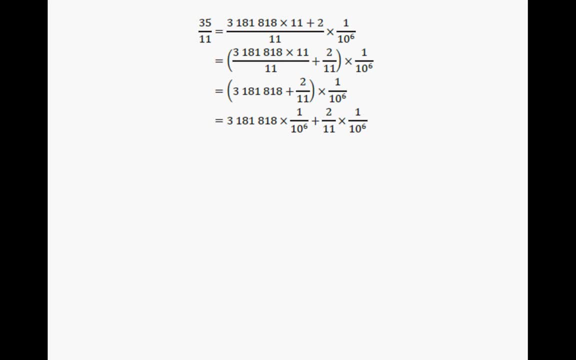 And then we're adding 2 11ths times 1 over 10 to the 6th power. This gives us 3,181,818 divided by 10 to the 6th power, plus 2 11ths times 1 over 10 to the 6th power. 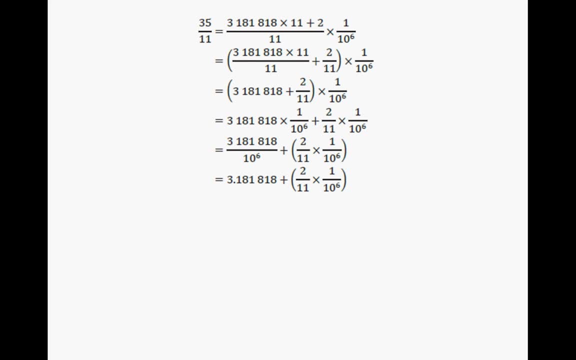 So, writing this as a decimal, we get 3.181818 plus the quantity or the product of 2 11ths times 1 over 10 to the 6th power. So at this point we have a fairly good estimation of the decimal. 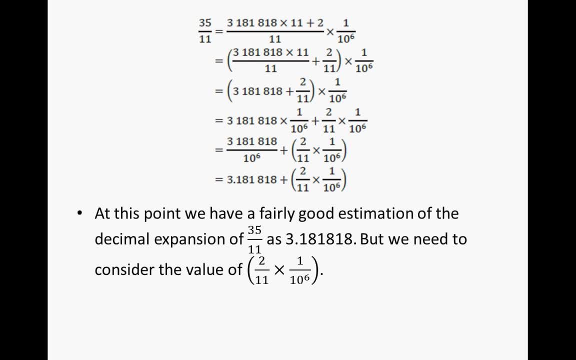 expansion of 35 11ths as 3.181818.. But we need to consider the value of 2 11ths times 1 over 10 to the 6th power. Well, we know that 2 11ths times 1 over 10 to the 6th power is 2 11ths times 1 over. 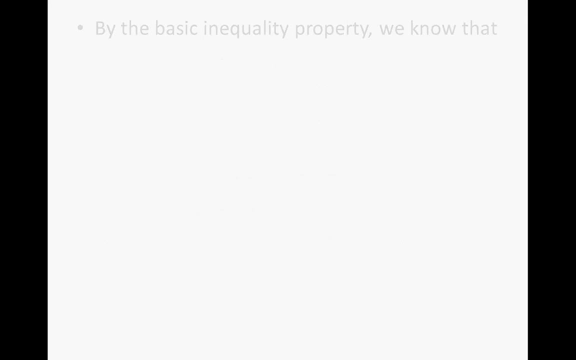 10 to the 6th power. So we know that 2 11ths times 1 over 10 to the 6th power is going to be less than 1 times 1 over 10 to the 6th power. So that gives us 2 11ths times 1 over 10 to the 6th power. 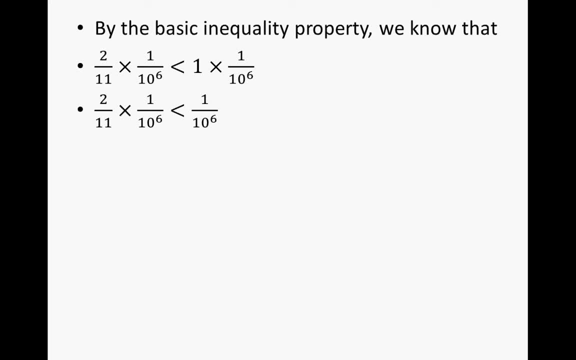 is less than 1 over 10 to the 6th power, Because again, multiplying that by 1 just gives us the same value And that means that the value of 2 11ths times 1 over 10 to the 6th power is less than 0.00001.. 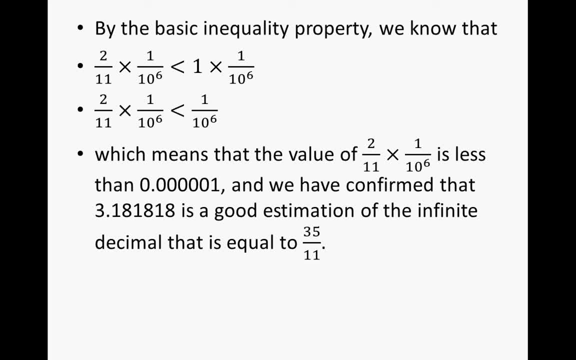 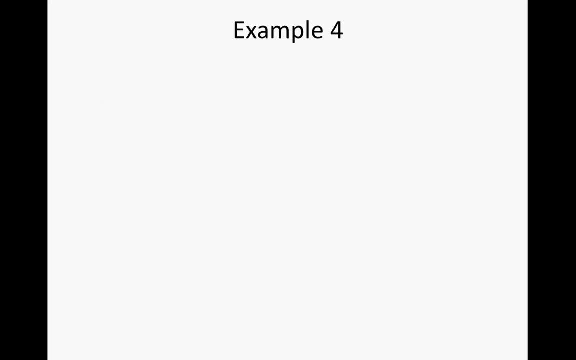 And now we have confirmed that 3.181818 is a good estimation of the infinite decimal. that is equal to 35 11ths. All right, let's do example 4.. Write the decimal expansion of the fraction: 6 7ths. 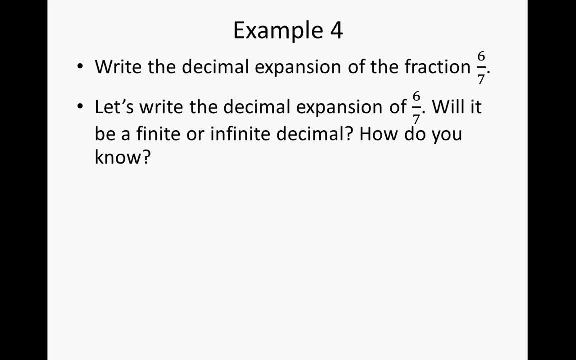 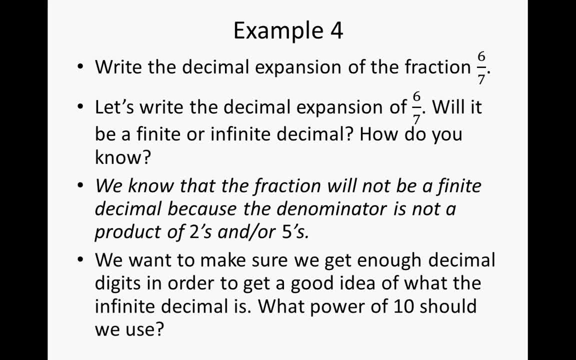 So we're going to write the decimal expansion of the fraction 6- 7ths. So we want to make sure we get enough decimal digits in order to get a good idea of what the infinite decimal is. What power of 10 should we use? 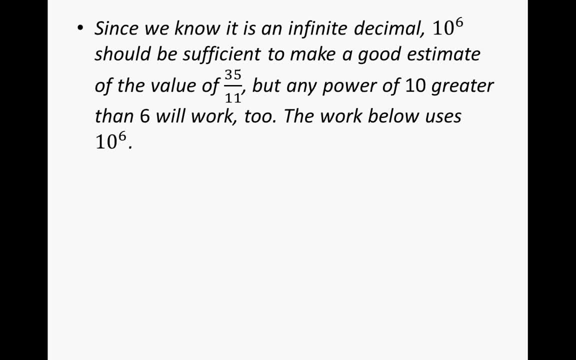 Well, since we know it's an infinite decimal, 10 to the 6th power should be sufficient to make a good estimate of the value of 35 elevenths. But again, any power of 10 greater than 6 will work too. 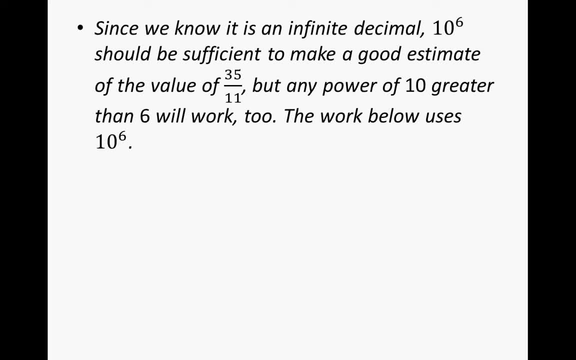 However, the work we're going to show uses 10 to the 6th power, And if you want to pick 10 to the 8th power, you can do that also. So using 10 to the 6th power, we have 6. sevenths is equal to 6 times 10 to the 6th power over. 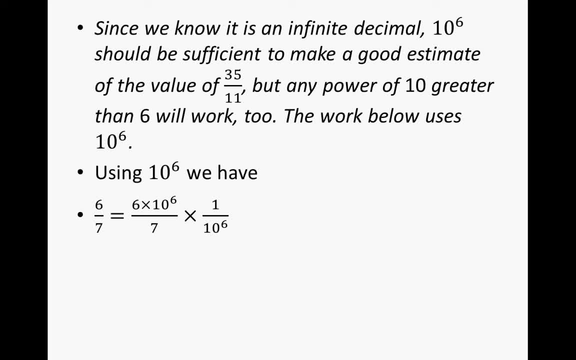 7 times 1 over 10 to the 6th power. And what do we do next? Well, 6 times 10 to the 6th power is 6 million. And then we need to do division with the remainder for 6 million divided by 7.. 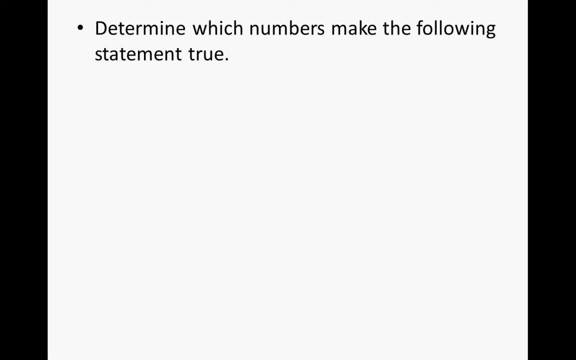 Okay, So determine which numbers make the following statement true: 6 million is equal to some number times 7 plus some number. Well, that would be 857,142, and 6 would give us 6 million equals 857,142 times 7 plus 6.. 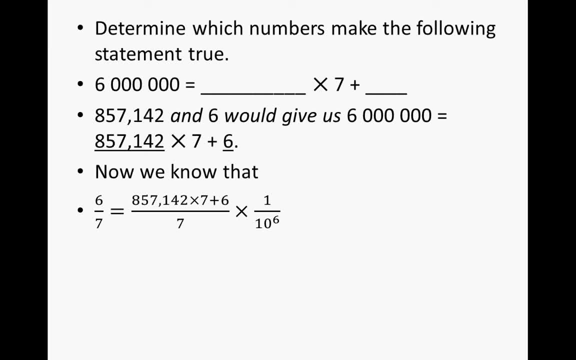 So now we know that 6 sevenths is equal to 857,142 times 7.. So now we know that 6 sevenths is equal to 857,142 times 7 plus 6 over 7 times 1 over 10. 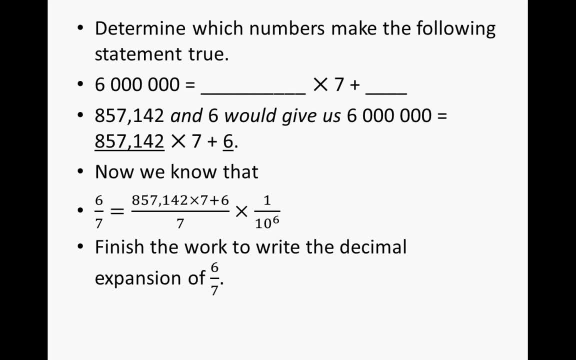 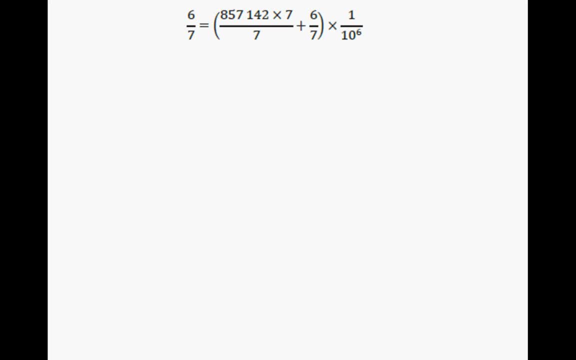 to the 6th power. So finish the work to write the decimal expansion of 6 sevenths. So, again following the same process- I'm not going to read this through, but you can just step through it- we get 857,142 plus 6 sevenths times 1 over 10 to the 6th power. 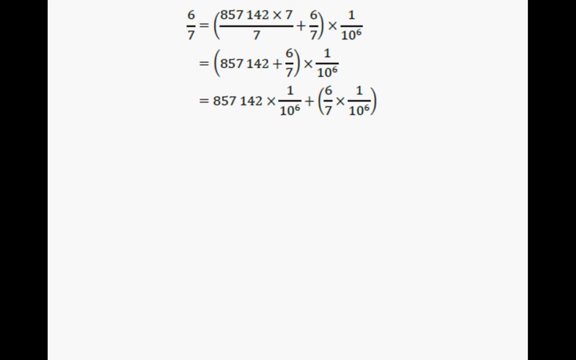 Then, by using distributive property, we get our two products, And by simplifying 857,142 over 10 to the 6th power, we get a decimal .857142 plus, and then the other product is 6 sevenths times 1 over 10 to the 6th power.